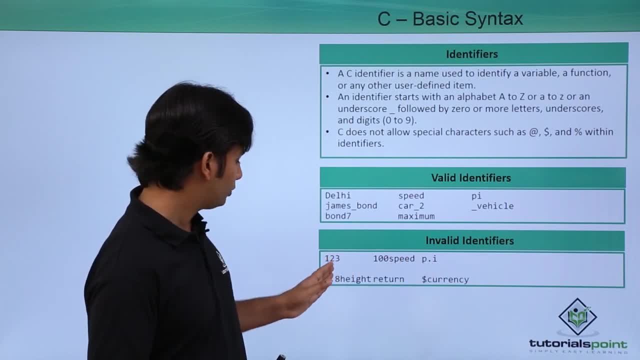 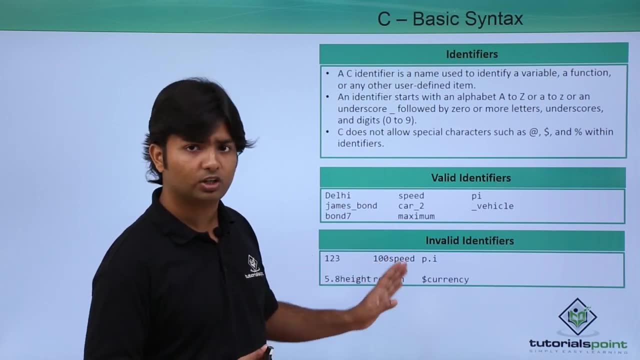 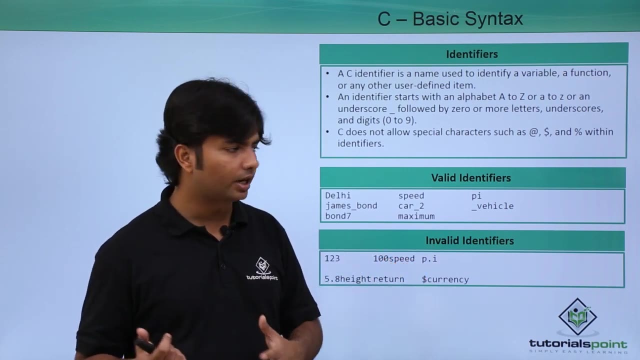 start a name with the number, like here: 1, 2, 3, 5.8 height. that should not be there. apart from that, there should be no space in the name. there should not be any special character like dollar or decimal. so if i talk about the special character, as i said, only underscore will be accepted. so 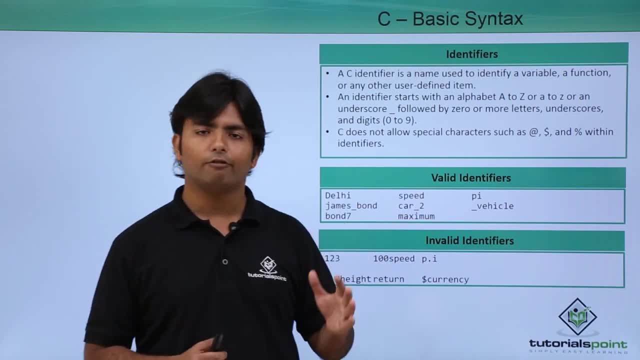 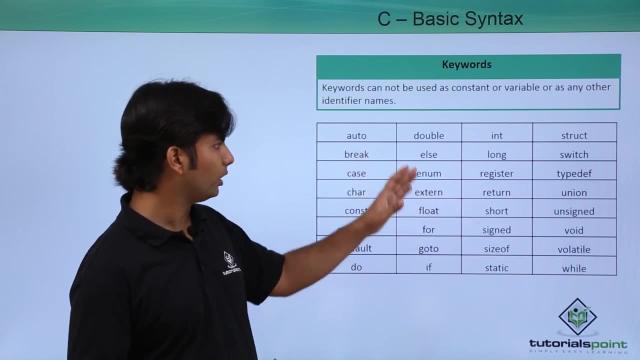 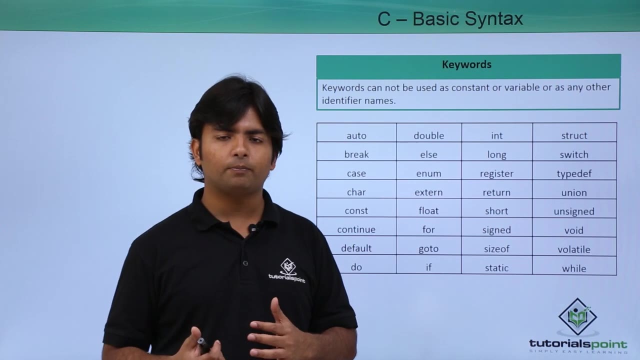 these are the basic things which you should keep it in your mind while giving the name to any identifier. now let's talk about some keywords. so in c language, we have 32 keywords which would be having some specific task. some of them are for the data types, some of them for returning. some of them 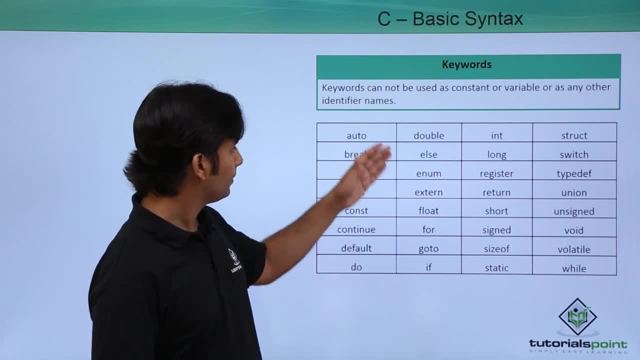 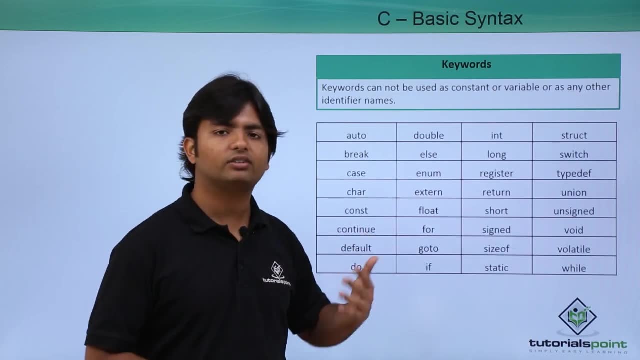 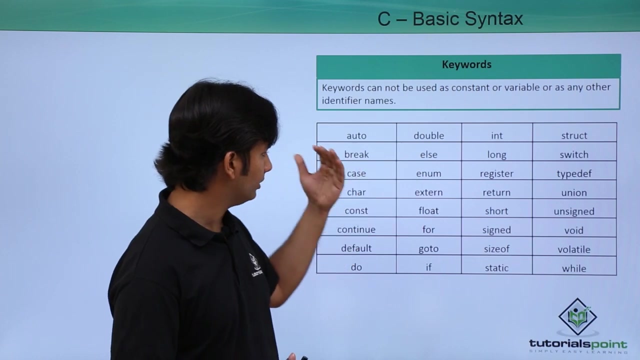 for the control statements like that, for example. here you can see, for is is a loop right if a statement do while. these are the basic control statement. similarly, you can also find the data type, like double integer, long float. so these are few things. so overall we have 32 keywords in c language. 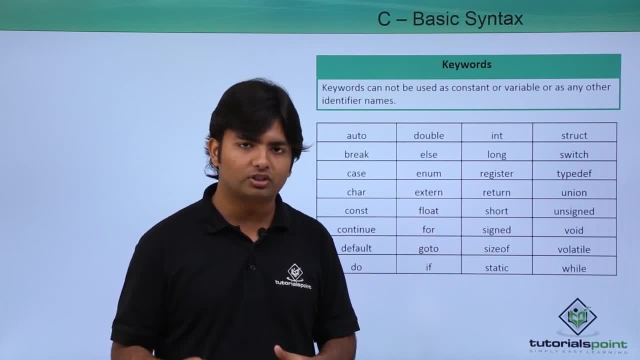 as we'll keep on proceeding, we will see the different usage of the different keywords. so these are the basic control statements, like that, for example. here you can see: for is a loop. so these are the basic control statements, like that, for example. here you can see: for is a loop. 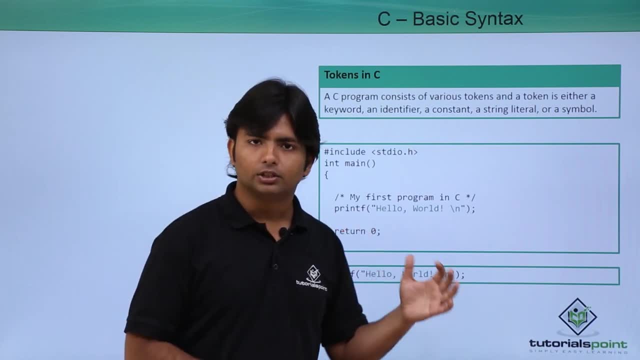 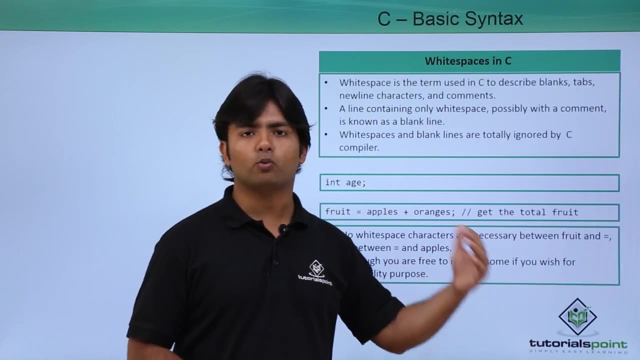 so in it is keyword, return is a keyword, so we will use such keywords for the different purposes. now let's talk about white spaces. white spaces basically used in order to make your code readable. for example, when you are done with one line after the semicolon, you press and enter for. 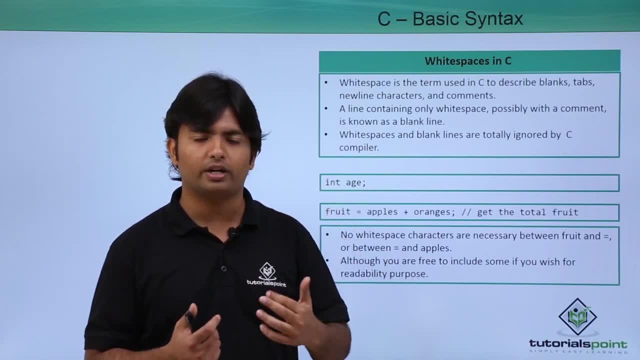 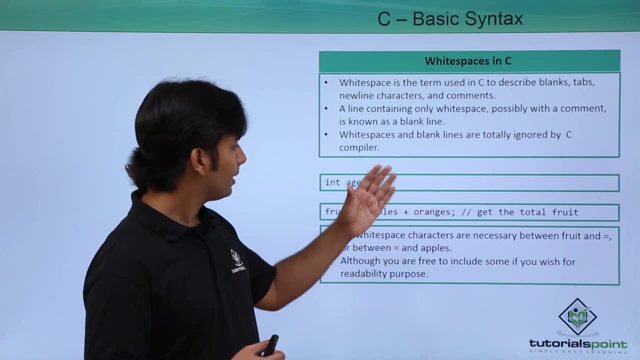 a new line so that when you will read, when any developer or any human will read the code, it will be easier for him to understand. similarly, you can also use the tab indentation in order to make your code more readable and more clear. as here you can see, fruit is equal to apples plus oranges here in between you.